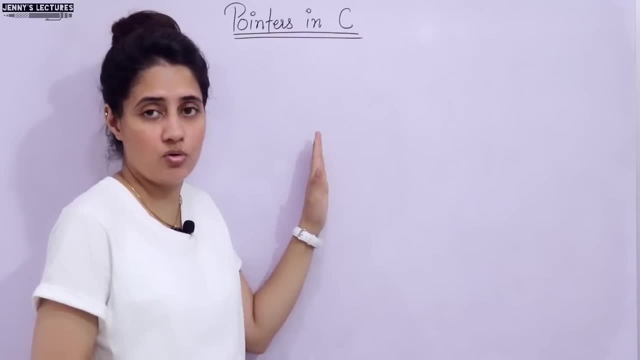 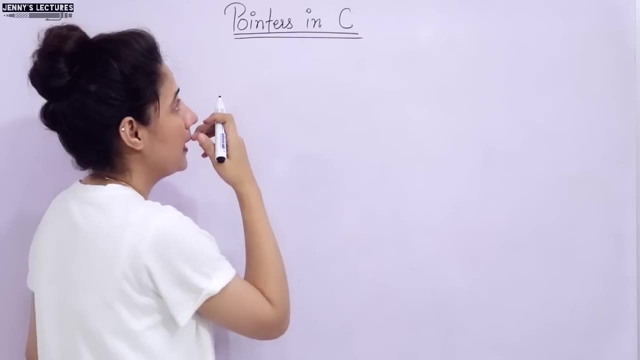 much in pointers. It is very simple to use pointers. you know concept right. What is pointer Before you know discussing pointer? just I just want to recap that thing. What is a variable? How to declare a variable? We have some fundamental a types in C like int, load. 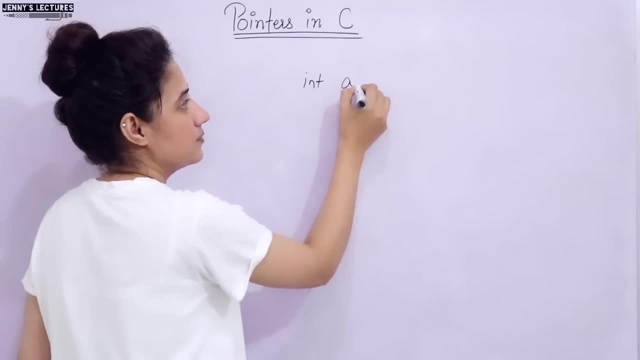 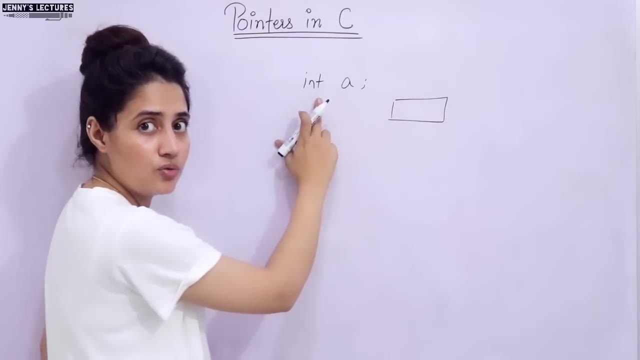 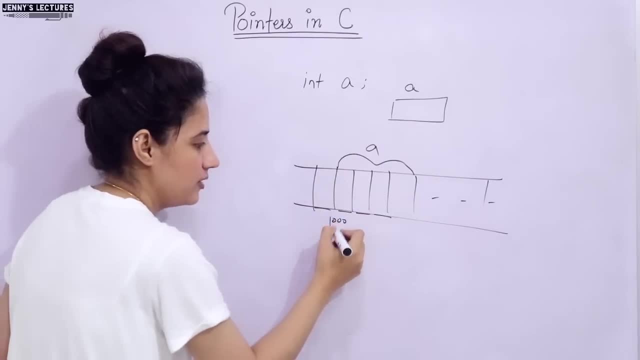 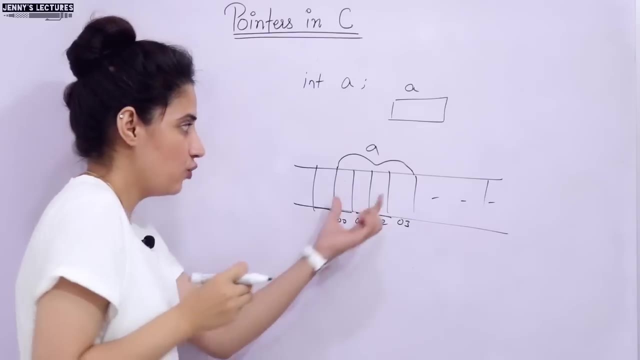 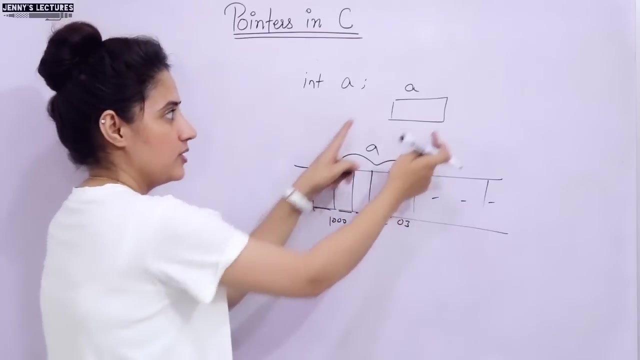 a Having some address, suppose thousand, first byte address, then this is thousand, then 1000, and one, two and three. These four bytes would be allocate to this a right. So I am not writing it something like this, I am just writing the four bits in a single. 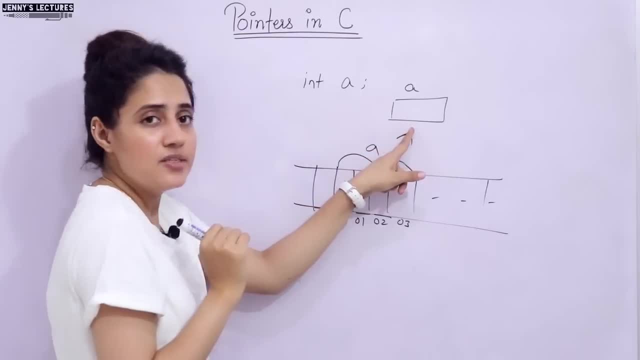 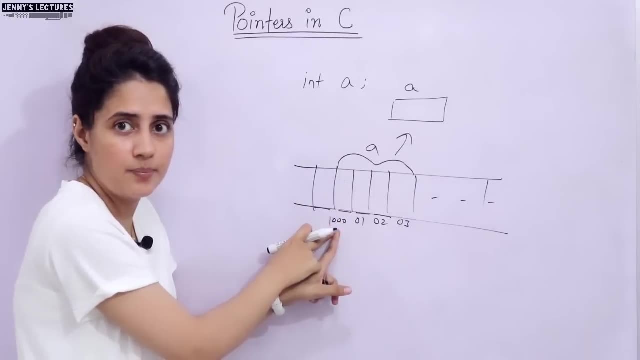 block, right? I'm writing it like this: And address is what, Obviously we will see. we will suppose the address of a is what Base address? Base address means the address of the first byte. that would be address of this variable. we consider it right. So address days. This is, since this yardsшие. 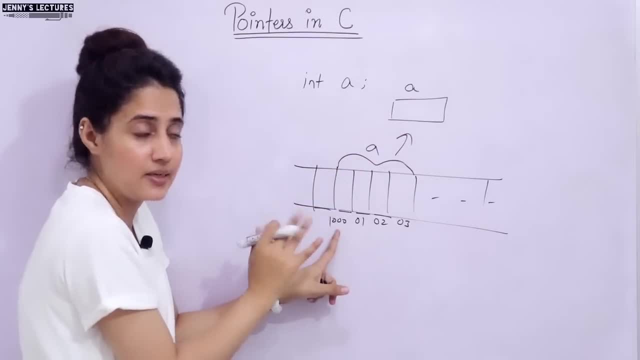 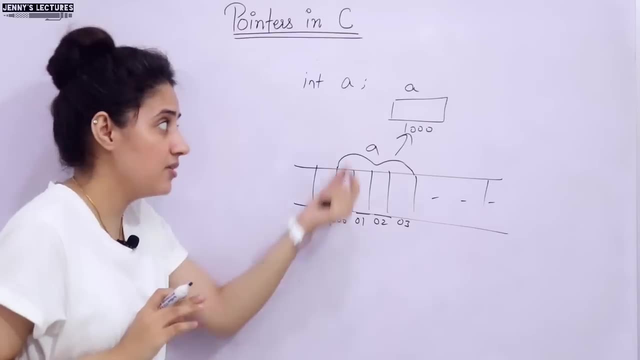 This is another Termine type variable itself. This means once we some address the data pieces is So: address is of ała be 1000.. From 1000 to 1003.. But we take base address that is 1000 only. So for simplicity, 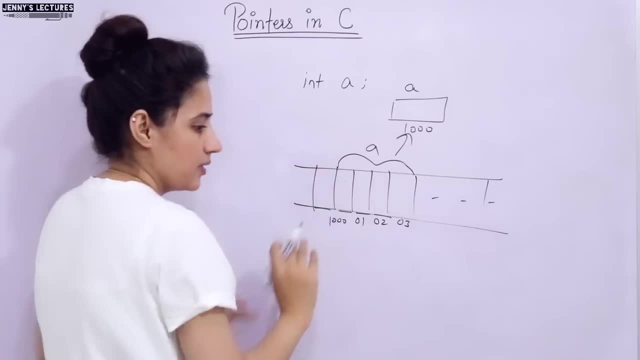 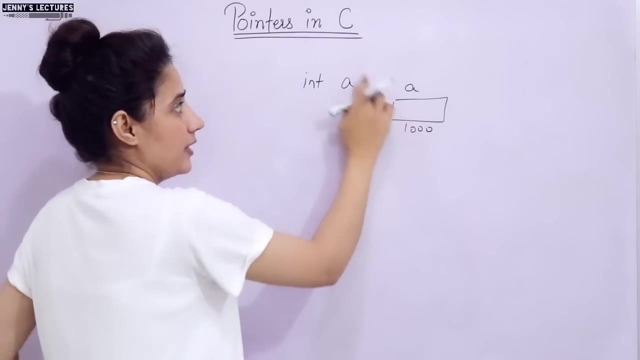 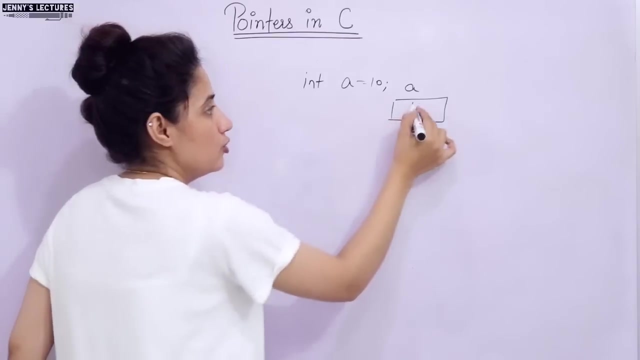 purpose. I am writing this something like this. I hope you got it Right. So now see this variable is having when. suppose I am initializing it. Now I am going, I haven't initialized it, So it is having some garbage value, So I am initializing, suppose it with 10 value, So 10 would be stored. 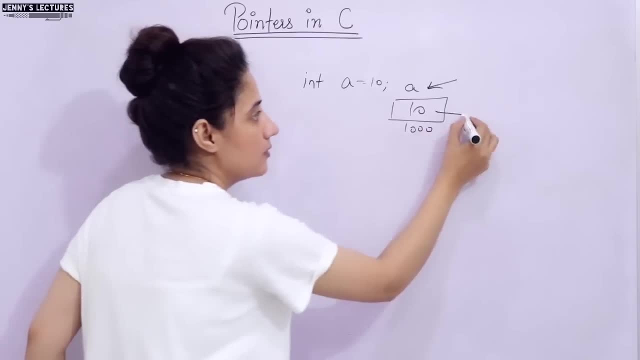 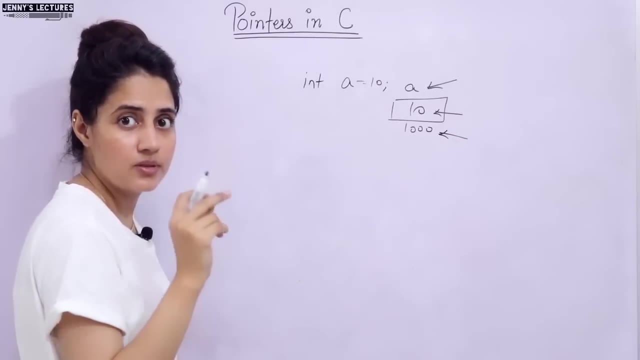 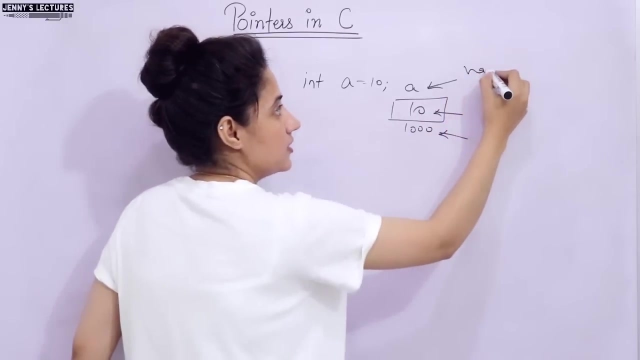 here. So this a is what Name of the variable, This is what Value of this variable, Right And this is what Address of the variable. Three things the variable will have: Right Name, value and address. This is name of the variable, This is what value And this is. 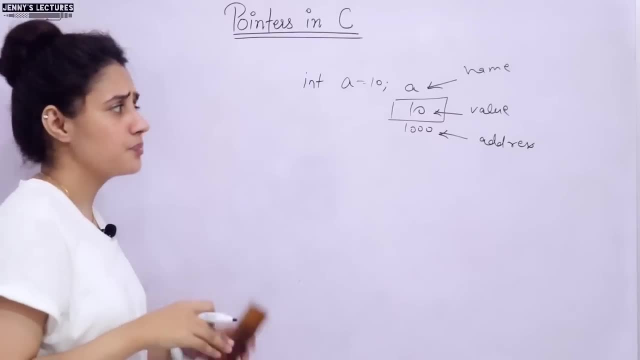 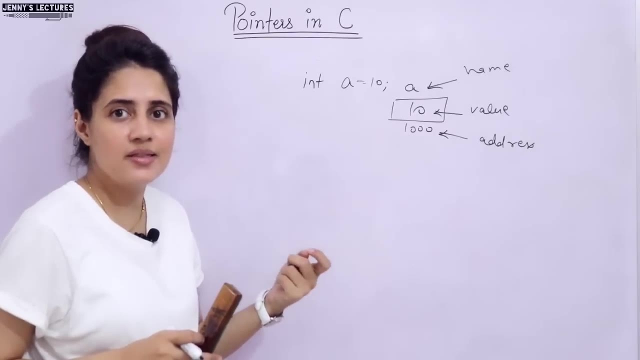 address of the variable. Right Now, pointer are also variables, Or we must say these are special variables. These are not these kind of variables. Pointers are special variables which contain address of any other variable. Right Pointer contains address of any other variable. 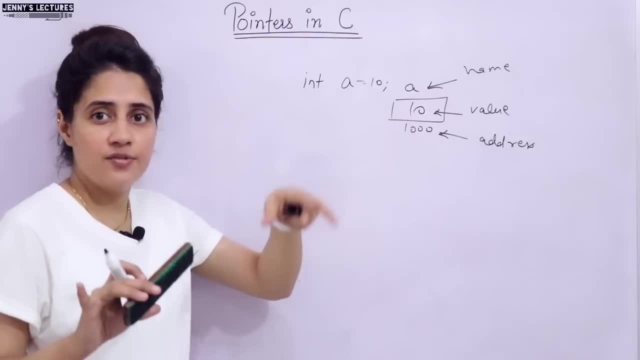 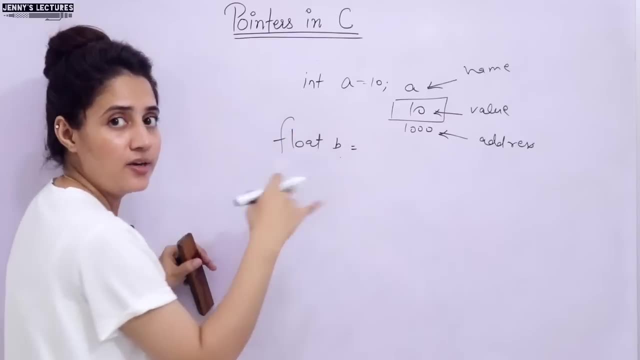 Pointer does not contain any simple value like 10, 5 or like integer value or float value, Float- if I take float variable like float b, it is going to take floating type of you know variable, So it is going to take floating type of variable, So it is going to take floating type. 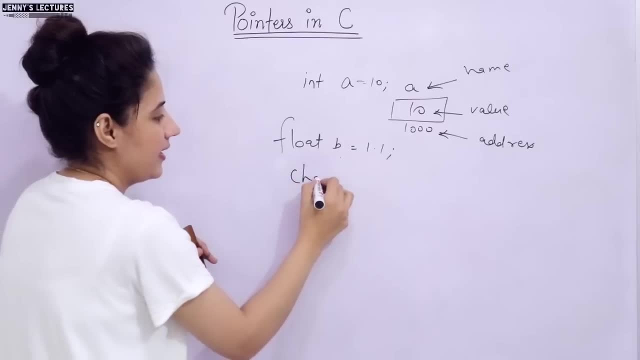 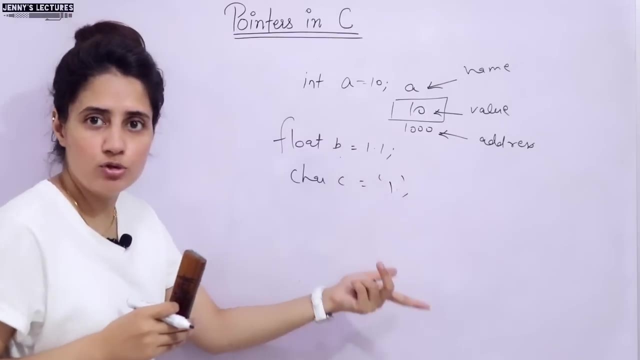 values like 1.1.. Right, If I take char, char, c, it will take character like a, b, c. or if I write 1 in single code, that is also considered as char. If I write 1, this is considered as integer. I hope. 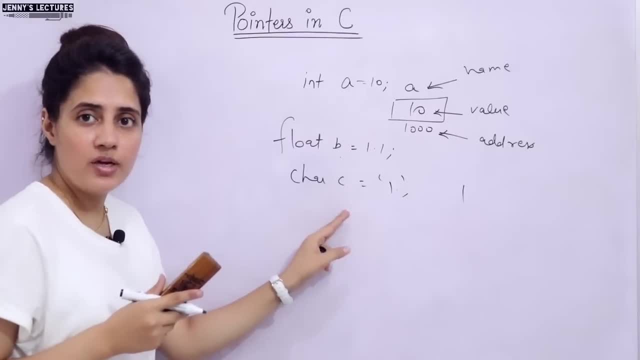 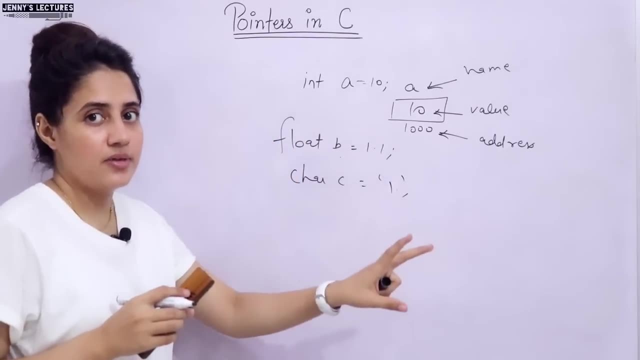 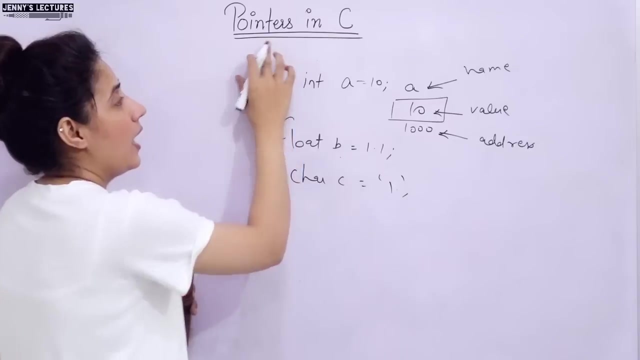 you got it Right. If you declare a double type of variable, that will contain, you know, double type of value. But pointer always contain address Address of any other variable, Right? So now see how I hope you got what is a pointer, or we can say pointers are derived data type. 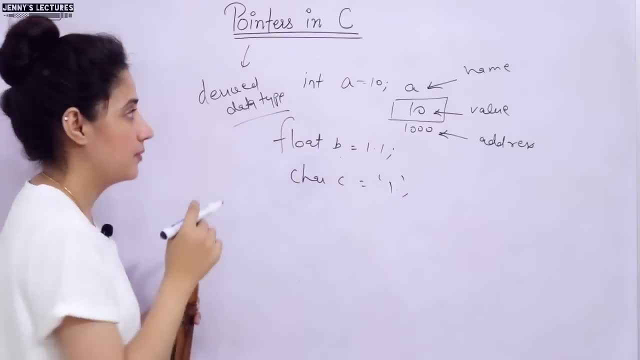 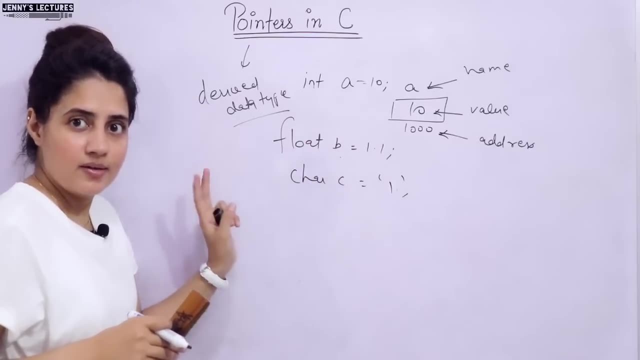 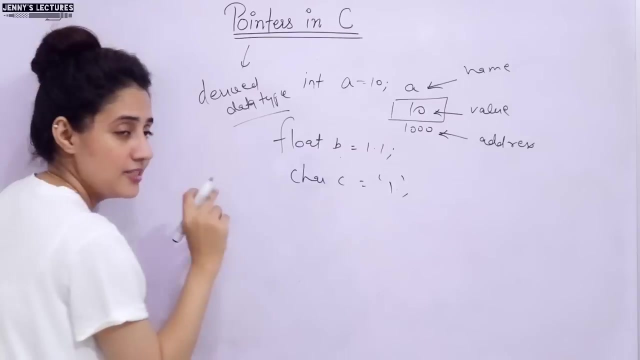 This comes under the category of derived data type, Right, Because we derive it using these fundamentals data types, Right. Fine, So now, how to declare a pointer? How to declare a pointer, See, this is. this thing is very, you know, important. This is very important, This is very important. 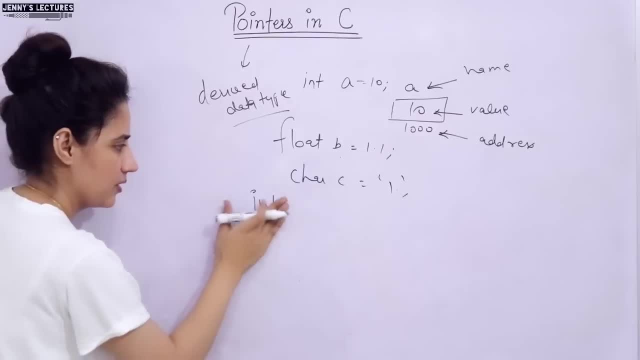 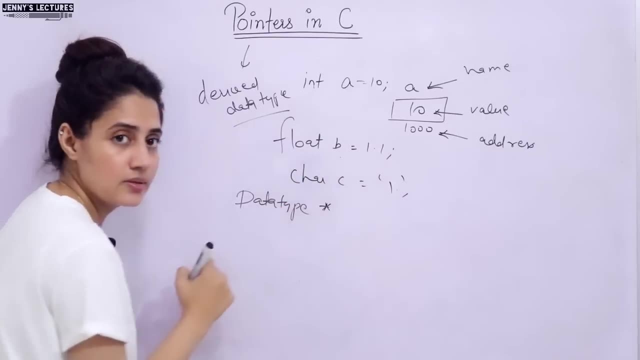 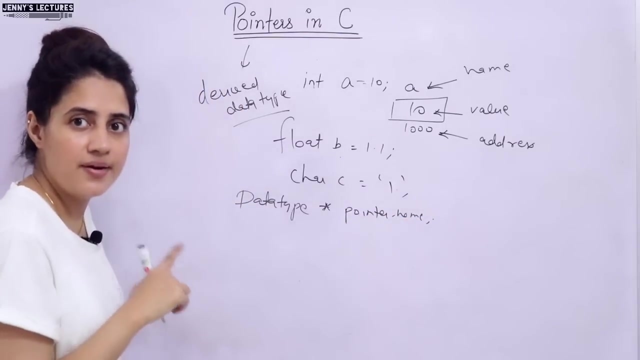 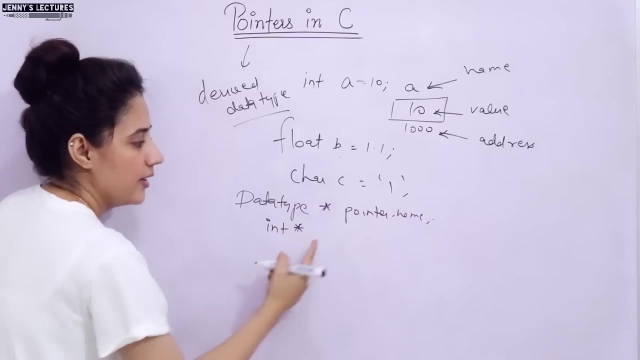 Please watch it carefully. If I write something like this, First we will write the generals. syntax should be data type, then asterix and then pointer name. This is general syntax to declare a right. So if I write here int asterisk and pointer name, I am taking, suppose, p. 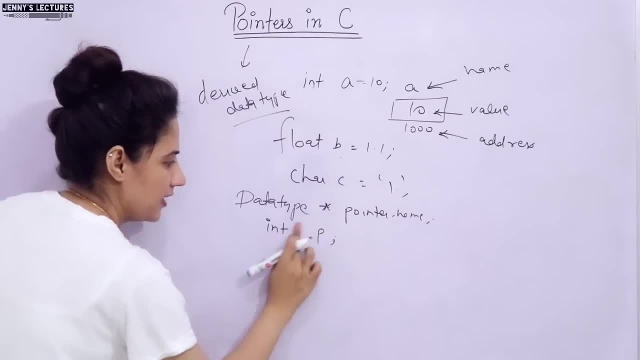 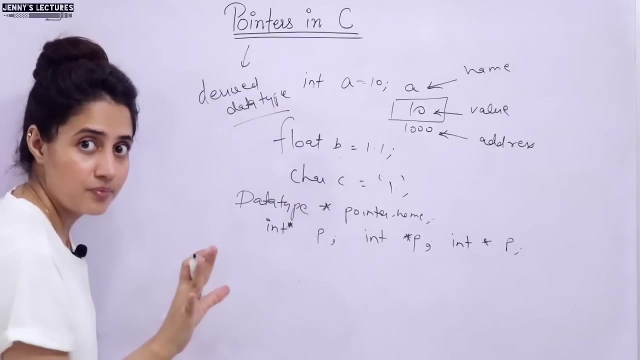 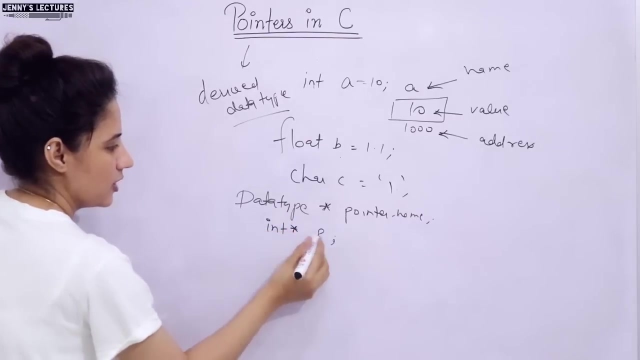 and see both. if you write this, something like this, like int- asterisk, this is also fine. if you write int- star p, this is also fine in c. if you write int- star p, these are same in c, right? So please do not get confused. I am writing something like this: int, then star and then p. 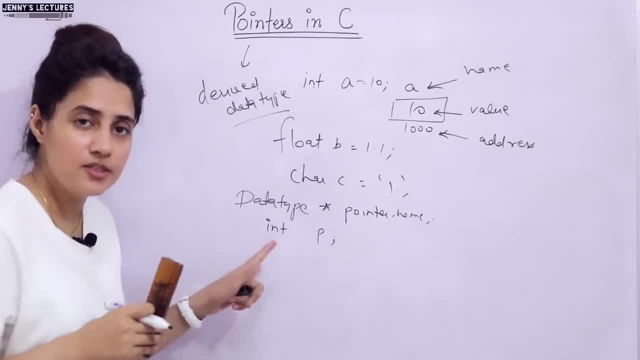 So now, if you write simply int p, it means p is a variable which will contain which type of value. int is a type of value, but if you write here this asterisk, it means p is what a pointer variable which will contain address of any other variable. 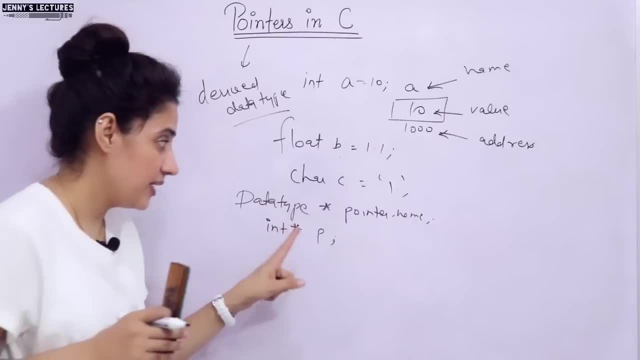 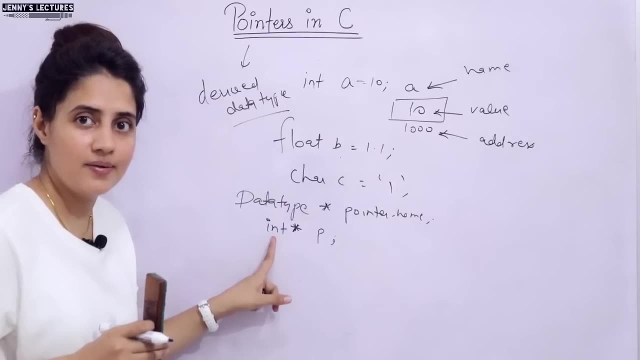 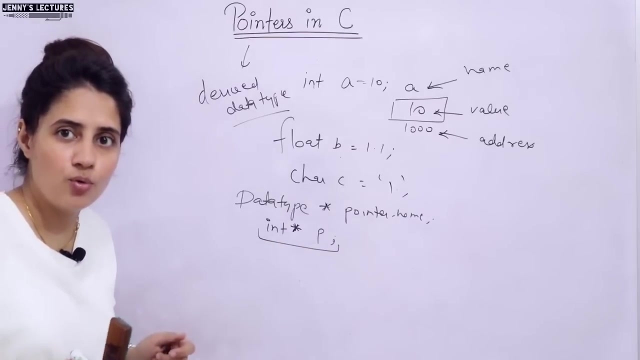 Right. And more specifically, if I say address of a integer type of variable, right, here we cannot say like the data type of pointer is int. no, if I write something like this, float asterisk p, maybe you will say data type of this pointer is float. here you will say data type of this pointer. 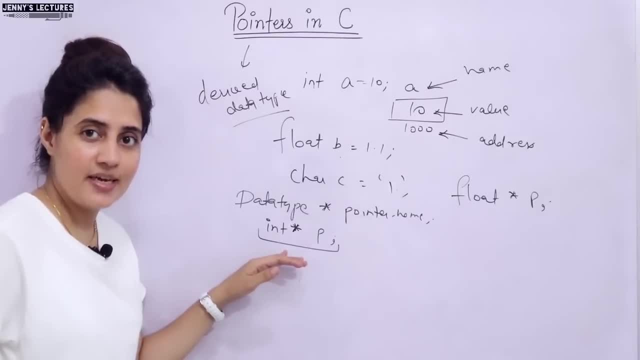 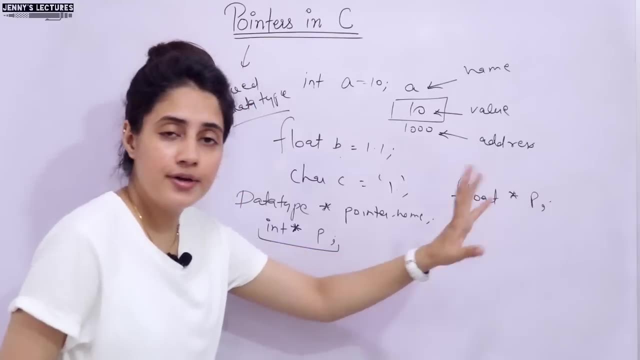 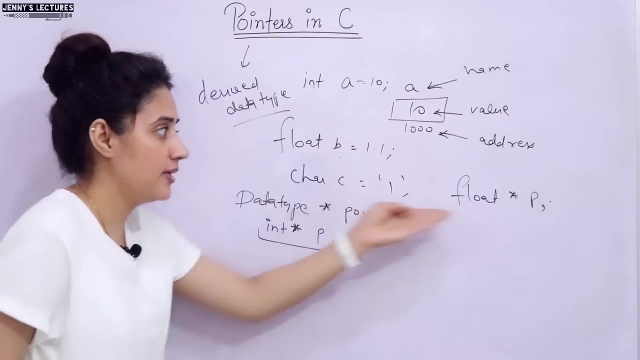 is int. This is the you know mistake many students do. but here here. here also pointer will contain address, here also pointer will contain address. right, in both the cases pointer will contain address. So how you can say: here data type is int, here data type is float, because pointer is. 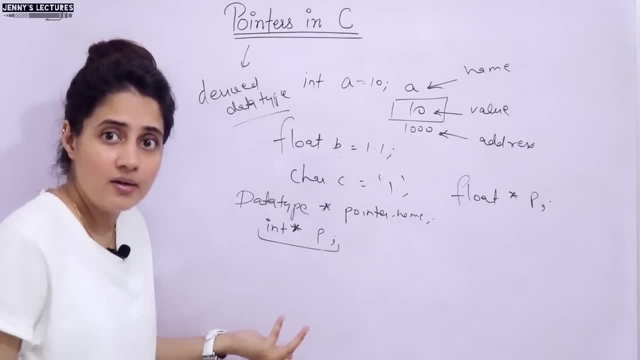 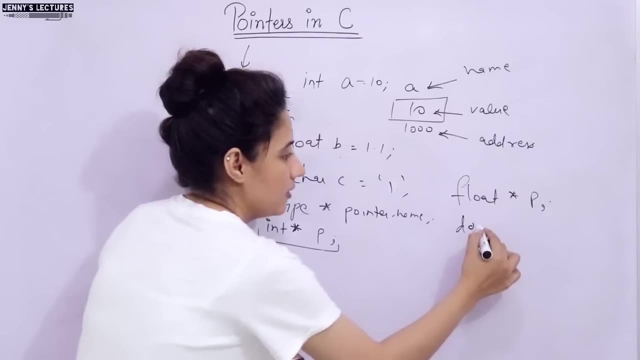 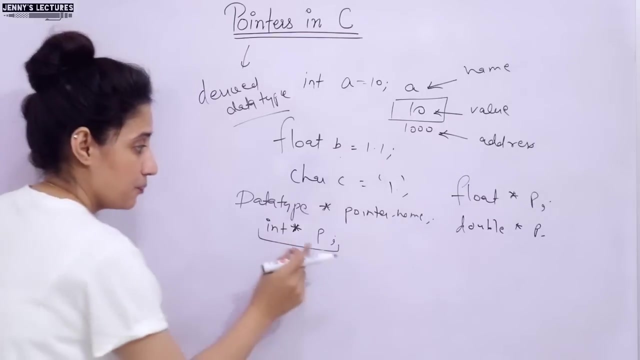 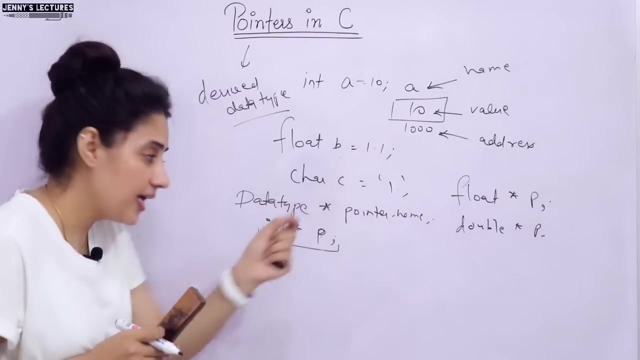 containing address, only right. So now, what does this data type mean? int float this. if I write here like double double star p, why I am writing the sin float double, It means here: this pointer p is containing address of a variable whose data type is a shot of. 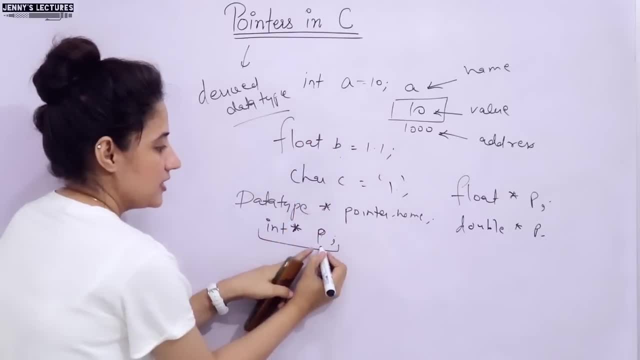 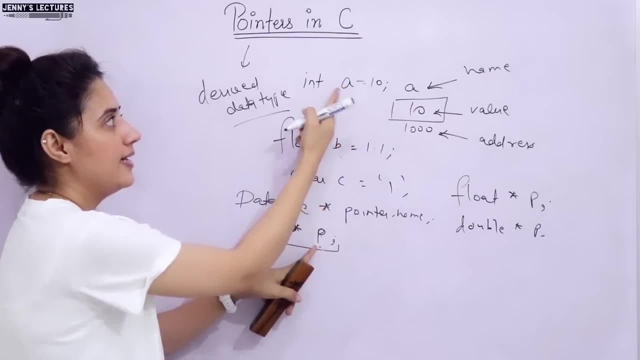 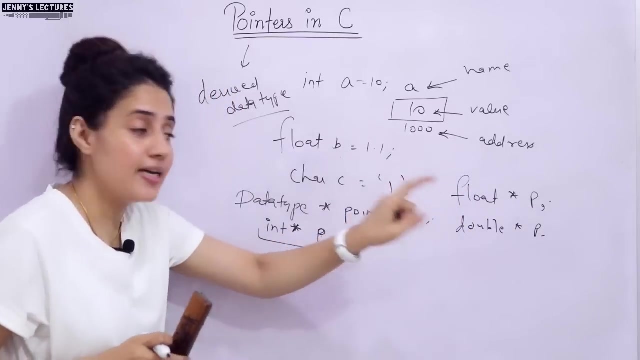 an integer right means here I can say p is containing address of a Like right, because see if you can say a, the data type of a is a shot of an integer. you can say this p will contain address of a variable whose data type is float. So p can contain here address of. 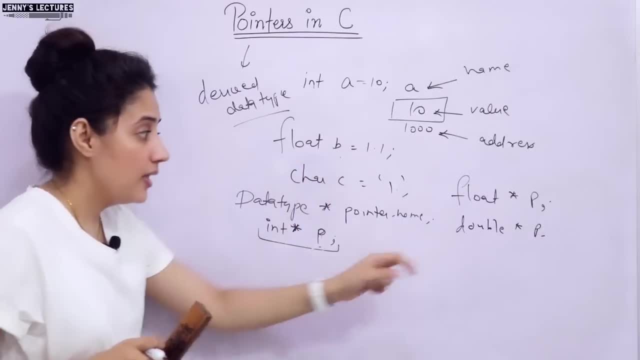 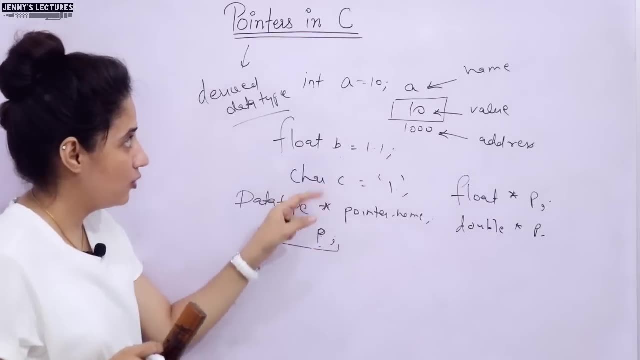 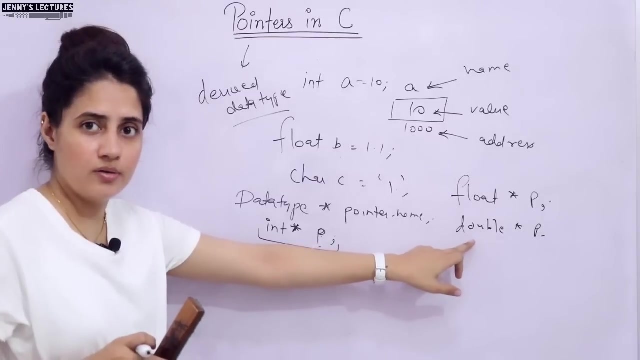 b because data type of b is float Here. p will contain address of a variable whose data type is double. I am not writing here double. If I declare double any you know variable there you can say: pointer will point: you know address of that variable. I hope you got like: why this? what? 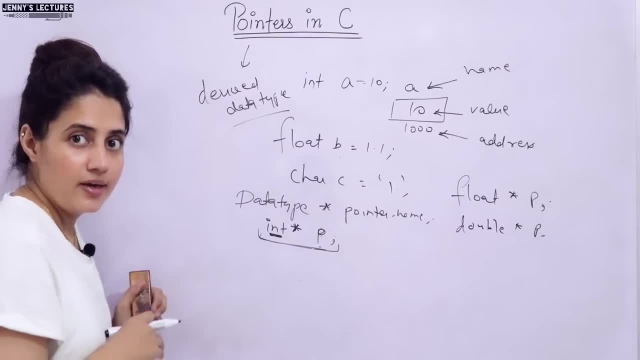 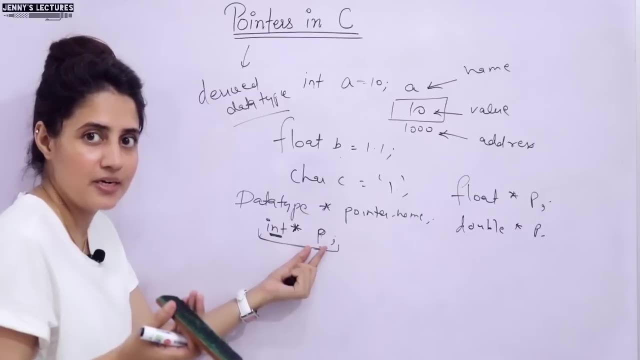 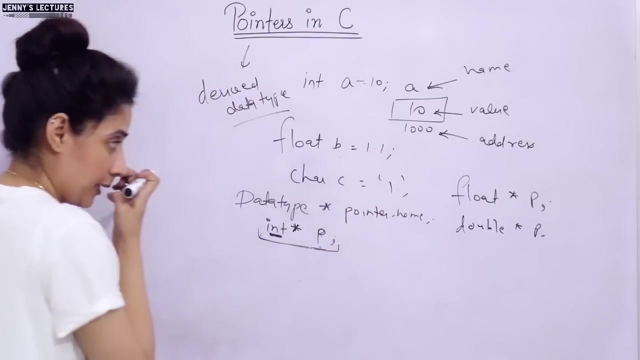 does this data type mean? right? So the size of pointer is what, 2 bytes for 32 bits machine? right, It depends, right. So now I hope you got the meaning of this thing and if you declare, if you write, So the basic, you know what is pointer. Pointer will contain address of any 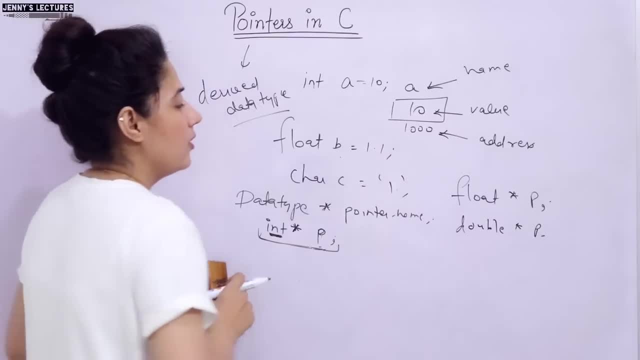 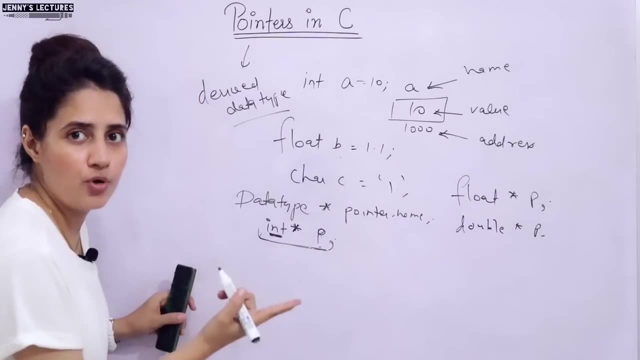 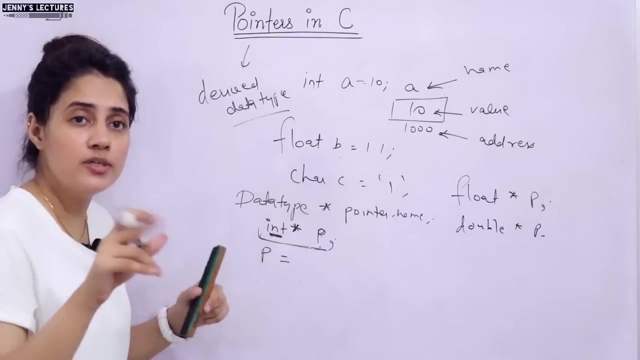 other variable. right. So now here, this is what declaration of pointer. Now here, what can I say? How to initialize a pointer. How to initialize a pointer p equal to now, p will contain address. and how we will get address of any other variable using address of. 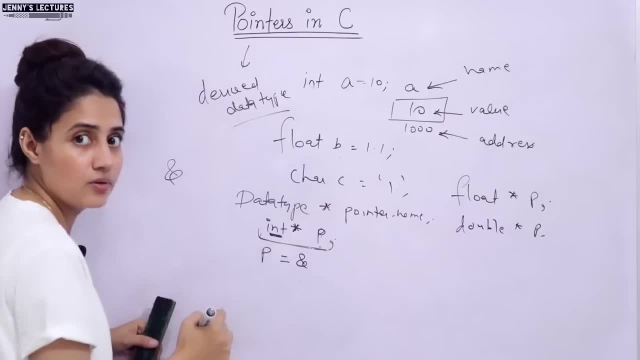 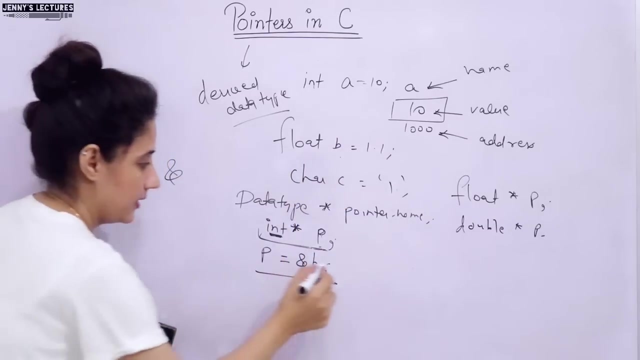 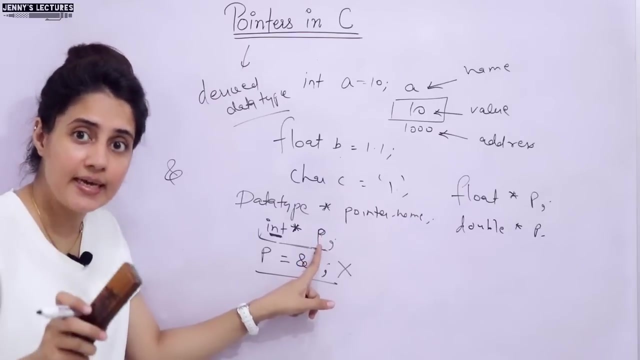 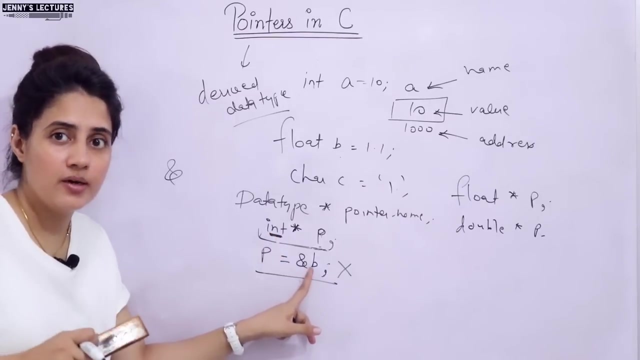 operator. So address of what I can write here, a address of a. See here, if you write, p is equal to address of b. It is not Correct. Why? Because according to the declaration of pointer, p should contain address of a variable whose data type is integer. But here I am initializing: p is equal to address of b. I am. 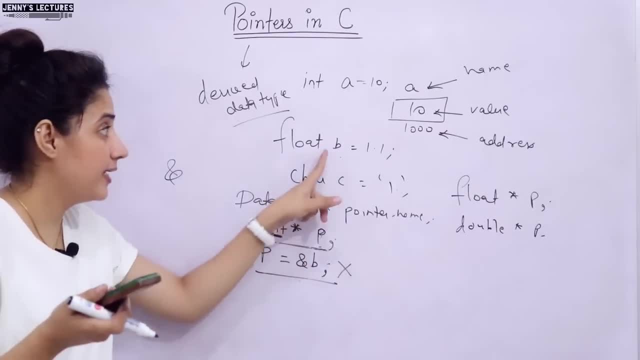 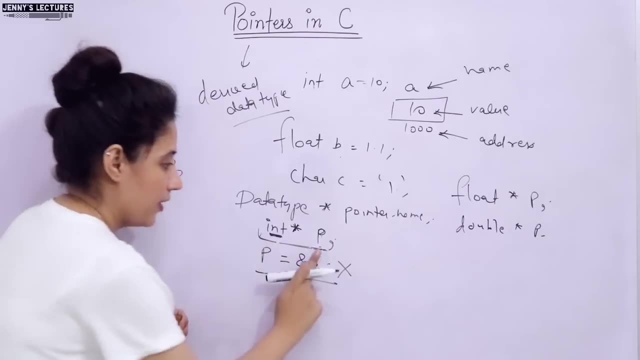 going to store address of b in p, But data type of b is float, So that would be illegal, right? This is not possible. So now here you can only write down a name of the variable whose data type is integer. So a is having. 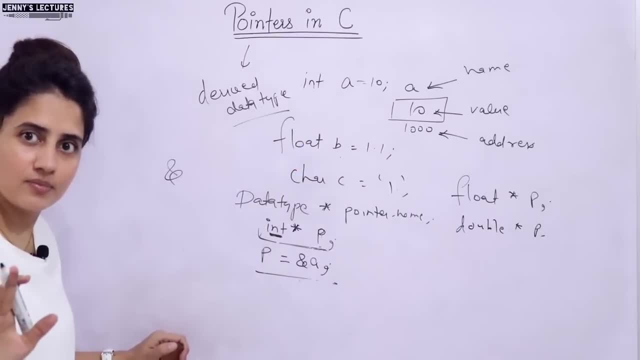 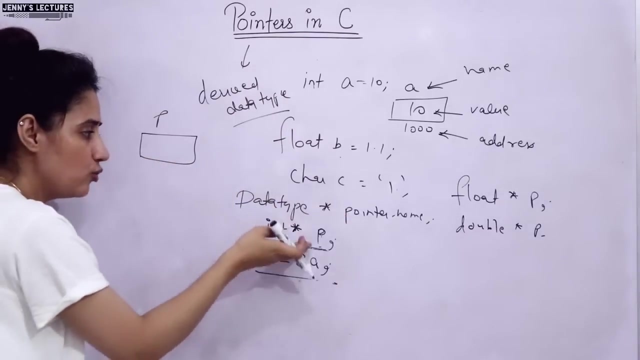 integer type. So that is fine, right. So now see, if you declare a pointer, something like this, then name: Obviously this is a variable, this is special variable which would will contain address. but this is also a variable. It is going to take some space in memory. Right, So here and if in memory. 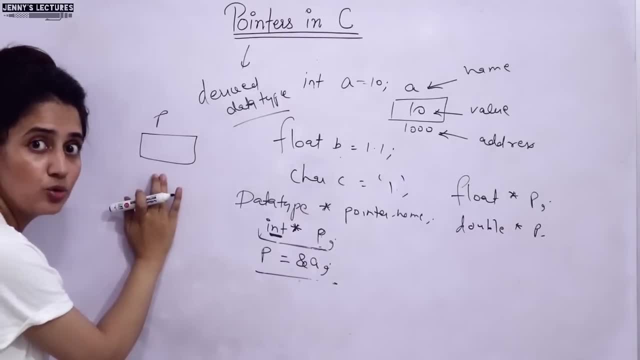 memory has been allocated to this piece. obviously this will have its own address also, Right. So address may be 2000.. See, this address would be in hexadecimal form, Right? But just for simplicity purpose I am taking these integers Right. So now I have initialized: P is equal to address of A. Now, 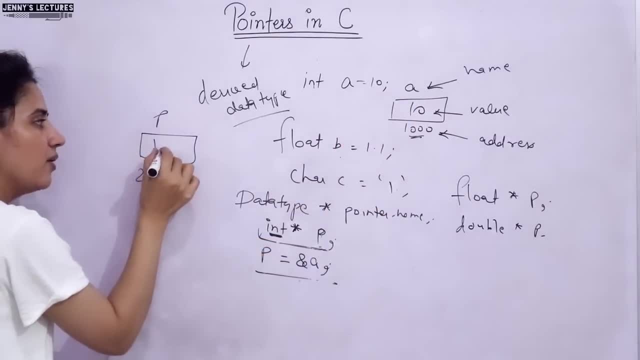 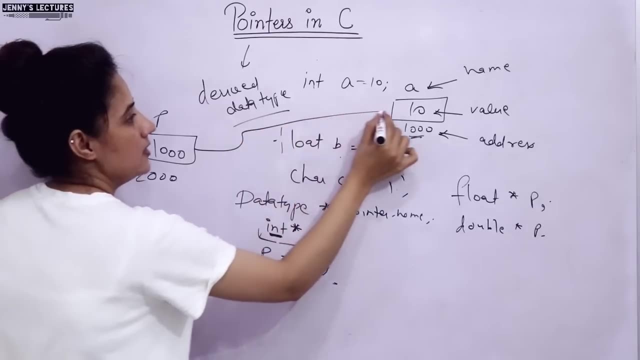 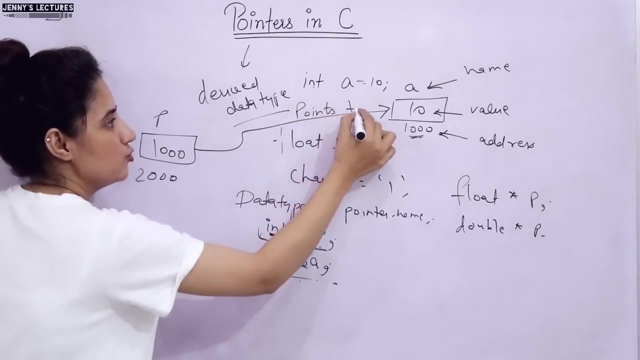 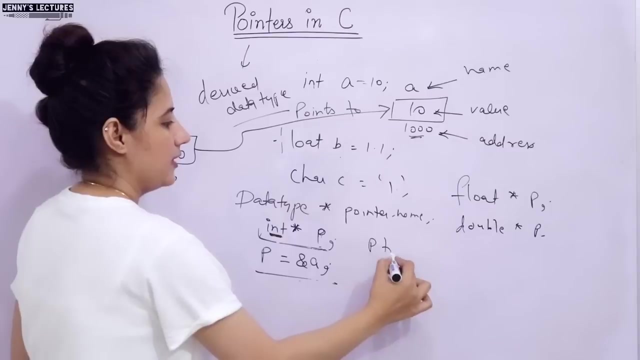 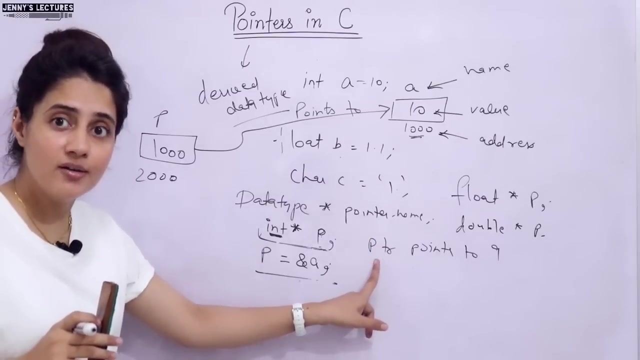 address of A is 1000.. So in P we have 1000.. So now what we can say, this P is pointing to A. Here we can write: P points to A If somewhere, somewhere, it is written like any variable name. PTR points to A Means definitely you will get. PTR is a pointer which is containing address of 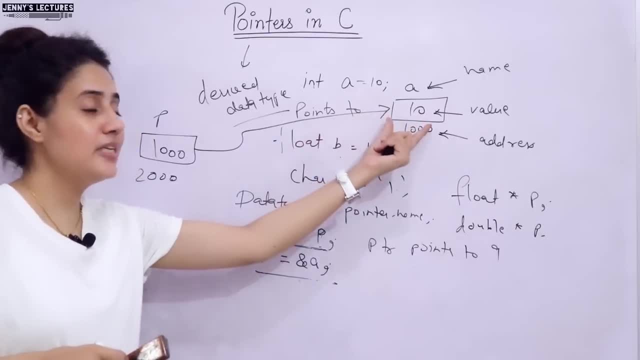 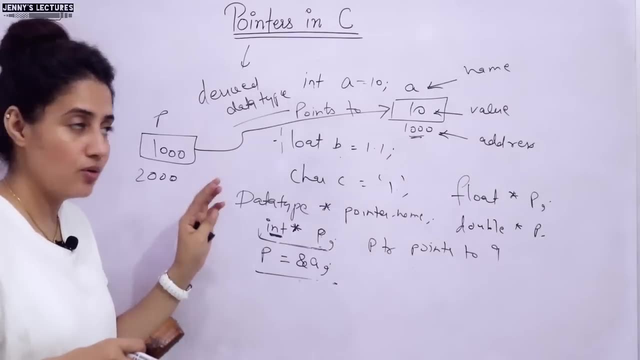 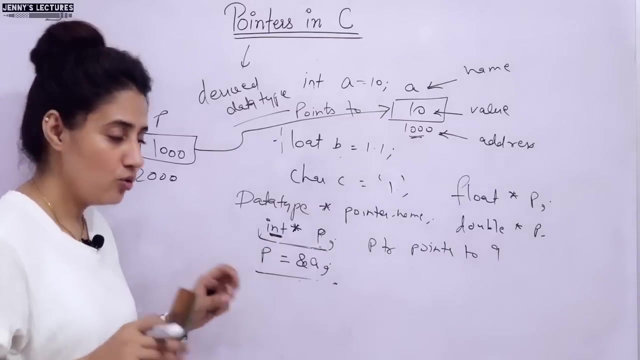 variable A Points to points to means it will. it is containing address of this A Right, I hope you got it. I hope you got the. you know the declaration and initialization of this pointer and what is a pointer Right, It is very simple. You do not have to be very you know, do not have to get. 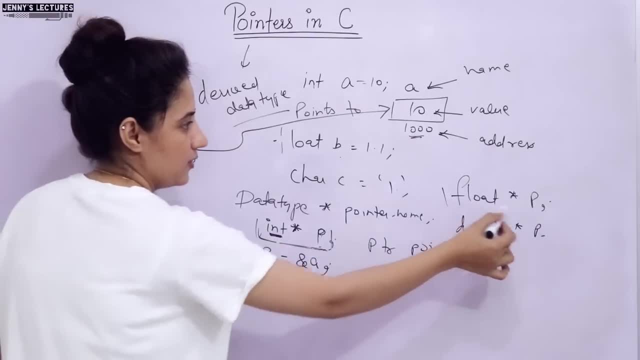 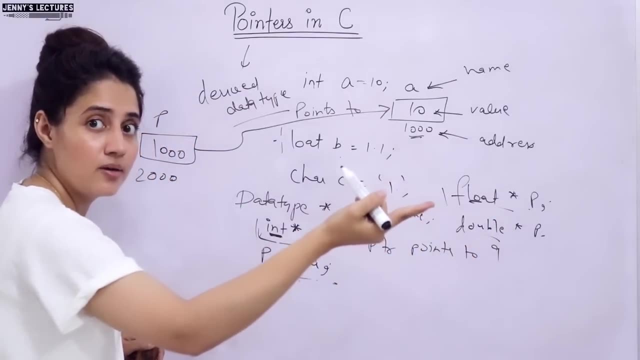 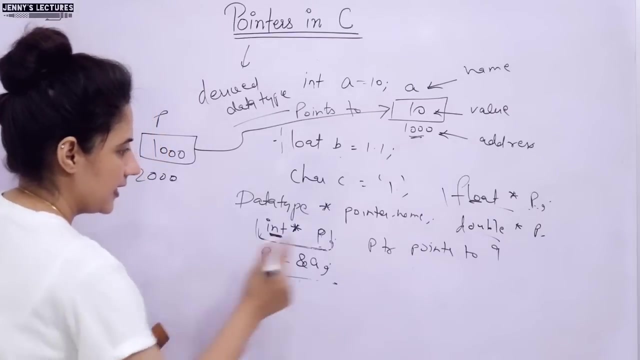 confused in this case. I hope you got meaning of this: int star P, float star P and double star P, Right, Please? it is not data type of pointer, It is data type of that variable whose whose address this pointer is going to store. Right, And this declaration, this is: 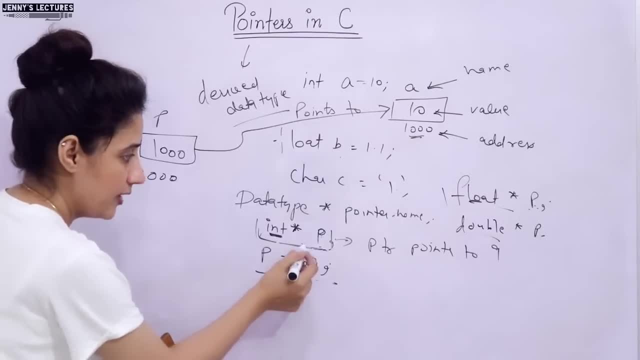 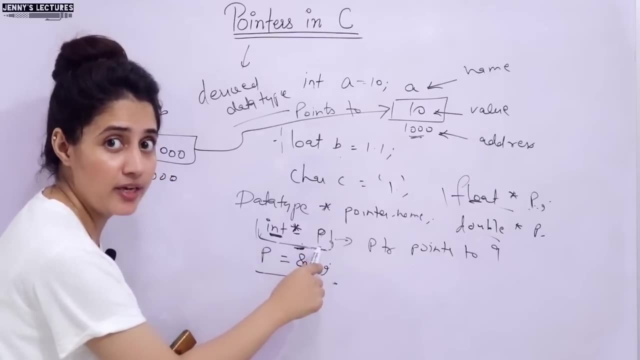 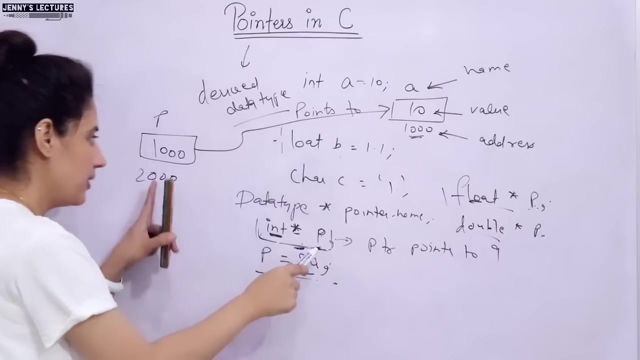 declaration of pointer. This is initialization of pointer, Right. So declaration is going to tell the compilers like three things: This asterisk means this would be a pointer type of variable, Right. And this P is having some space in memory, some address in memory, like 2000, maybe 2000.. 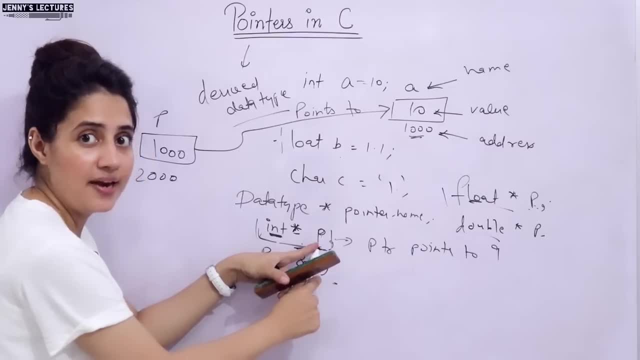 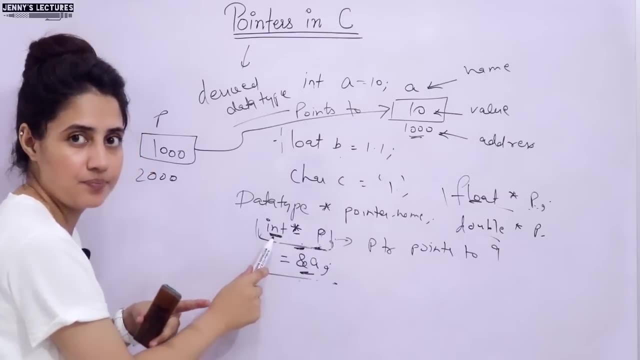 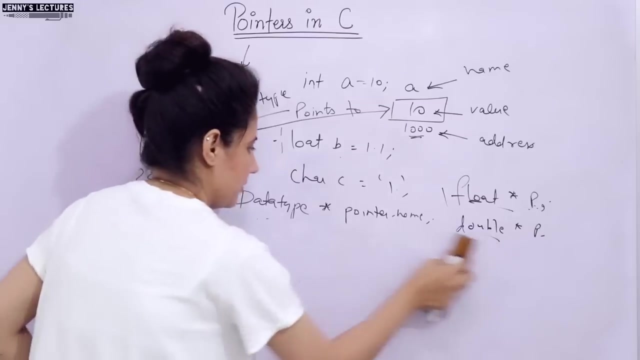 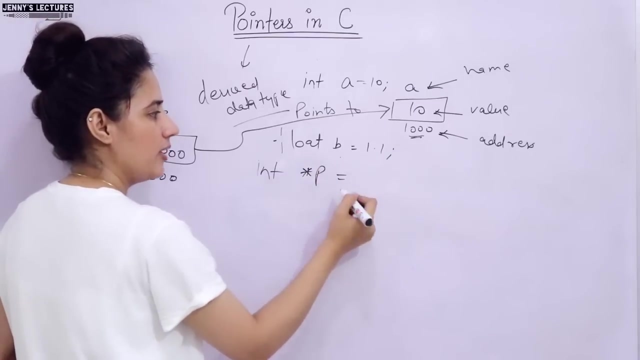 Let us suppose 2000.. Third thing is this: this is having address of a variable whose data type is integer. So it is having address of integer data type. Right Now you can do this declaration and this initialization in same step, Like I can declare something like this: Int star P, and here only I can say, is equal to address of. 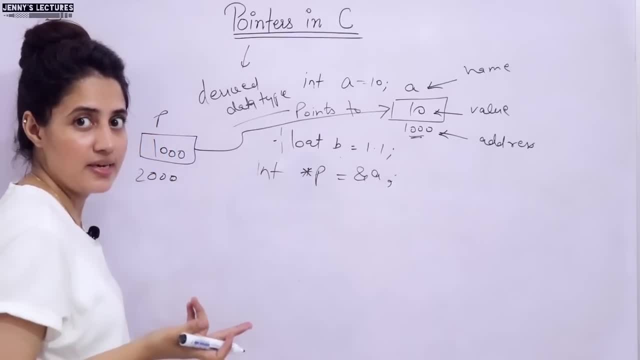 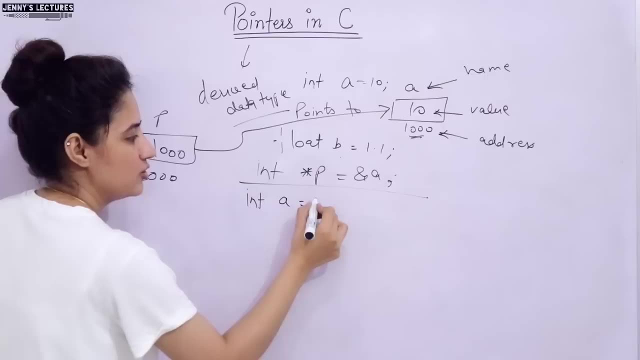 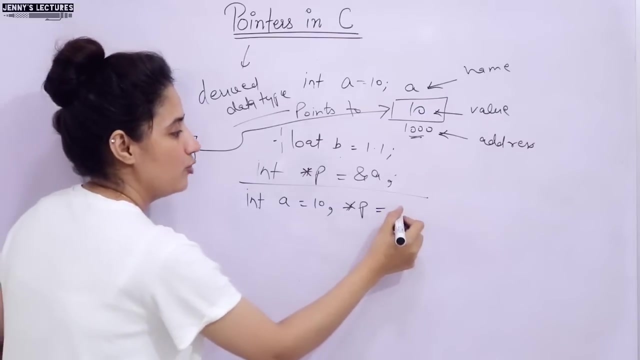 a. That is also fine in the same step. Or this is also fine: You can merge this and this in one line also, Int a is equal to 10. in the same line, I am going to declare a pointer star P and I am going to initialize it. address of a. 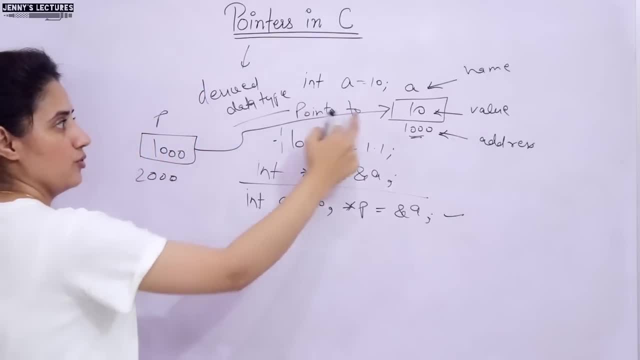 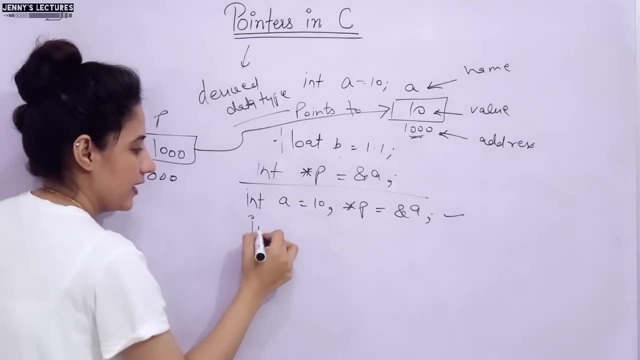 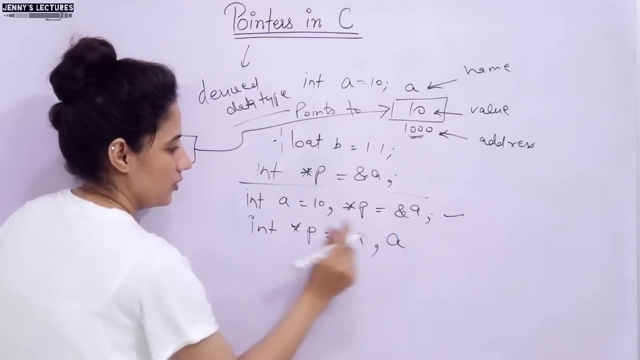 This is also fine. This will also, you know, points to this thing Visualize. you can visualize this thing, something like this, Right, But this is not correct. If you do something like this, int star P is equal to address of a, and after this I am going to initialize this: a: a is equal to 10.. 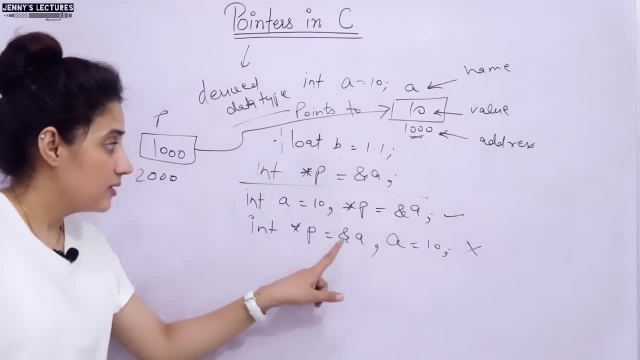 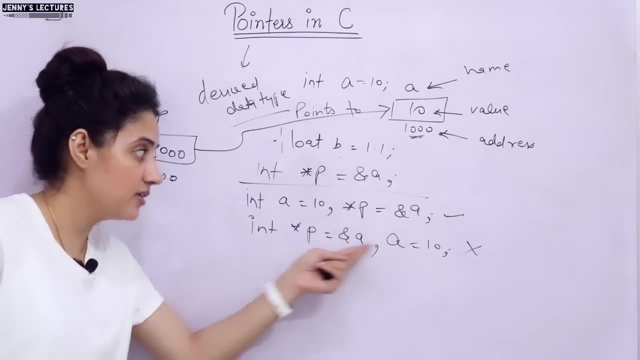 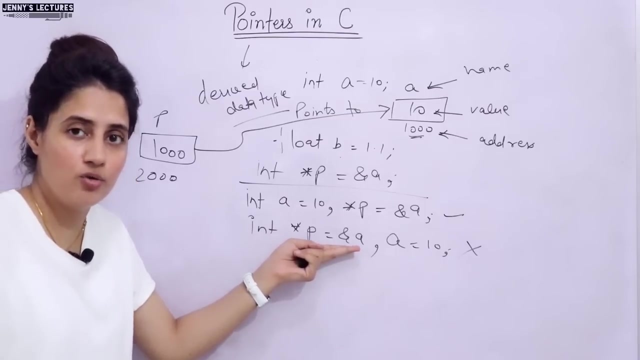 This would be wrong. Why so? Because we are. you are going to store address of a in this pointer, But you haven't declared a yet. You are declaring a after this. So where is a Here? till here, we don't have any a value or a. 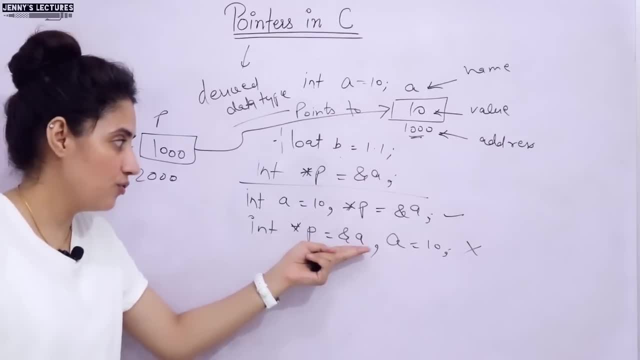 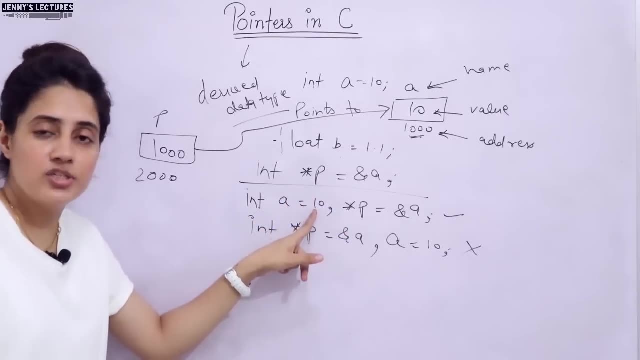 variable name in memory Right Any address of a in memory. So this would be illegal. But yeah, this is possible. First declare a or you can say: initialize this. You can also initialize it, or if you don't want to initialize, then it will contain any garbage. 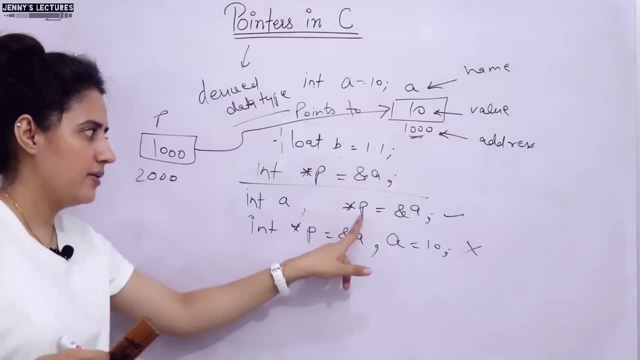 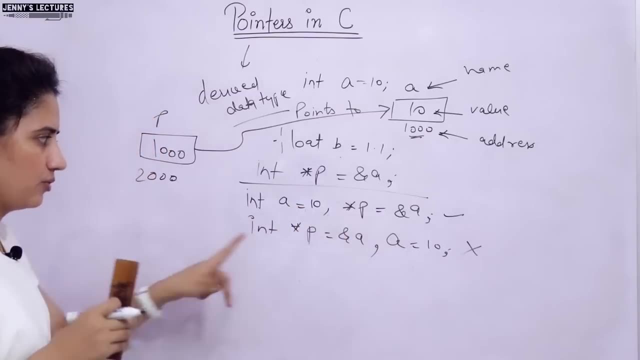 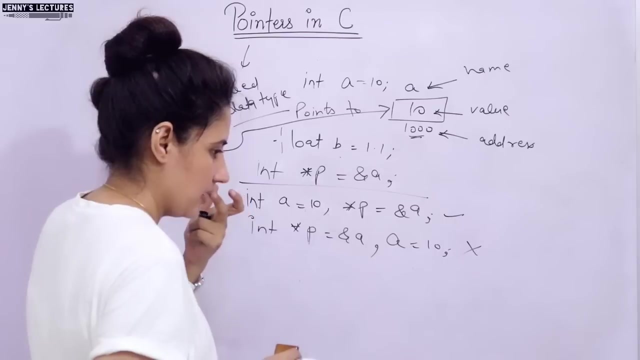 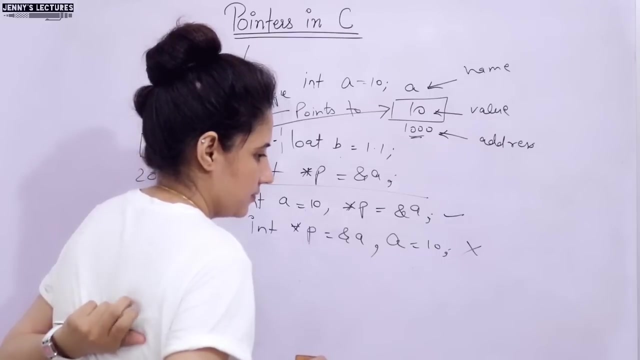 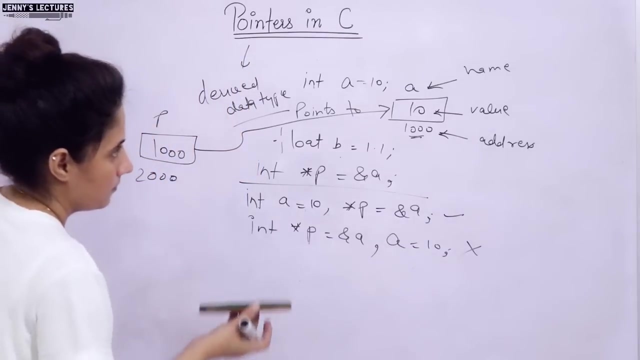 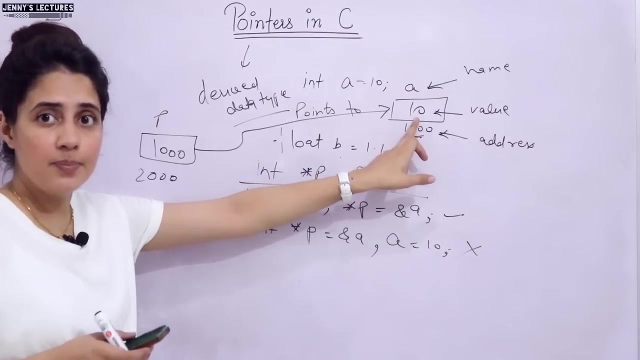 That is also fine, Like int a comma and star P is equal to address of. that is also fine. Right a will contain any garbage value, But this is not. you know, this would be illegal, This would be wrong, Fine. So now see, Uhh, Now we have two ways to print the value of a. You can directly print, print Mayor. 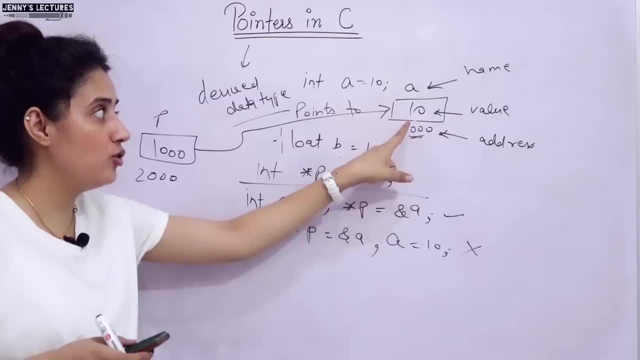 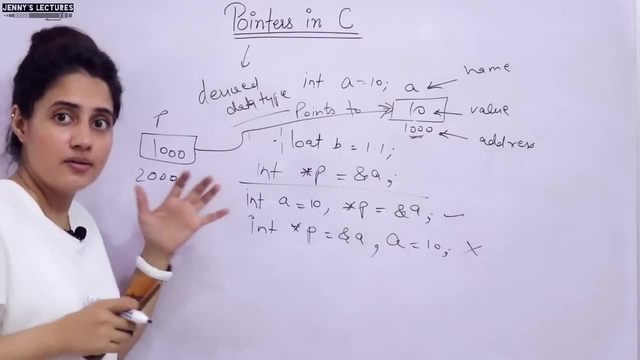 Toast A, %d and A, and you can also print the value of a using this pointer, because this pointer is also pointing to here. But how you will print the value, how you will access this value using pointer, There we have to use some special operator that is dereferencing operator Or it's. 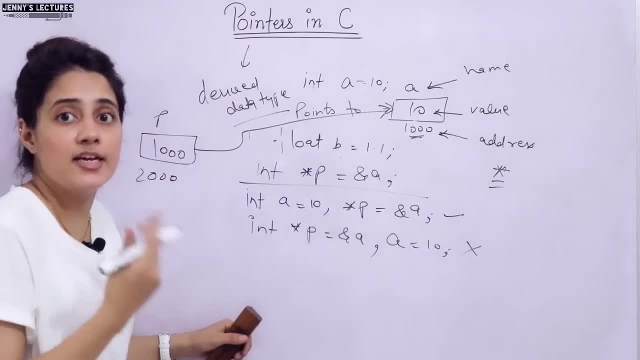 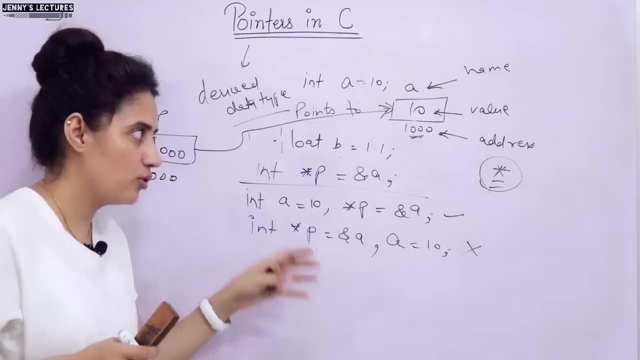 a bad interpreter, But here D is there, Are you able to get it? Well then, d is the Frequency of ФД, dereferencing operator or indirection operator, this star that we'll discuss in next video, right with some proper example, and i'll show you that program on my laptop also here i just, i just want. 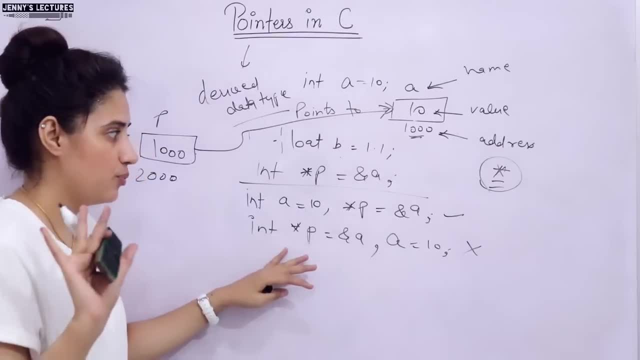 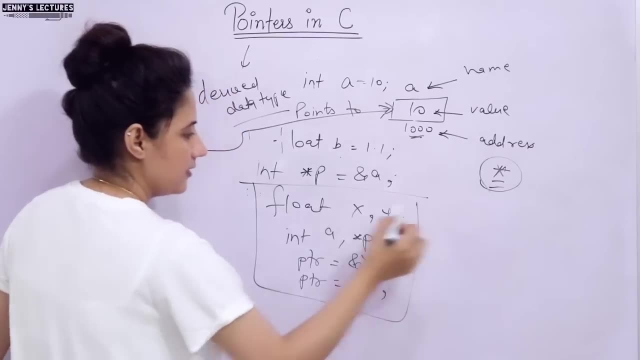 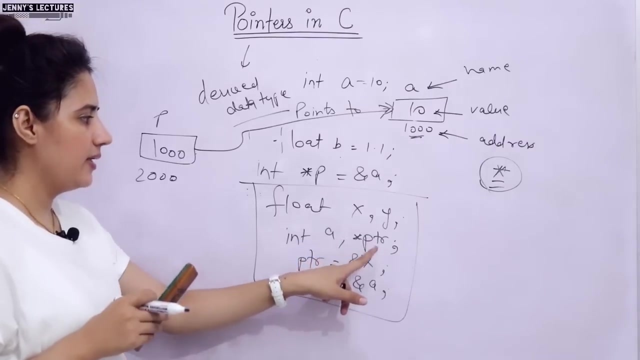 to you know, get you familiar with there with the basics of pointer right now. one question for you is if i write something like this, is this correct? you have to tell me in comment box right, two variable of type float x and y, one variable, int a, a pointer, and in pointer i'm storing address of. 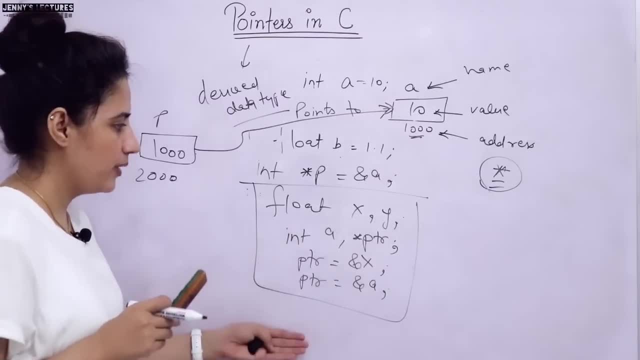 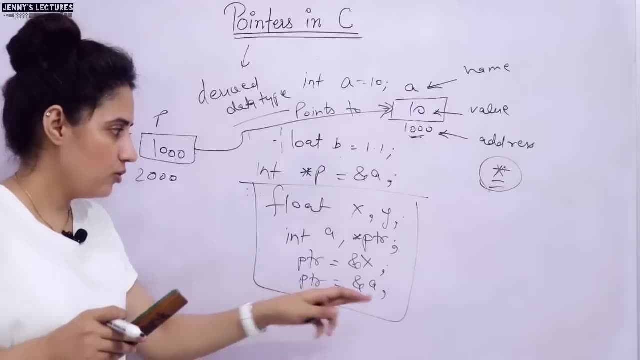 x and then address of a. i'm storing right so which would be correct and which maybe which would be wrong, and if both are correct, then at last in pointer, what would be the value? you can take any you know address, obviously you will take up to you thousand, two thousand, anything right, and then you 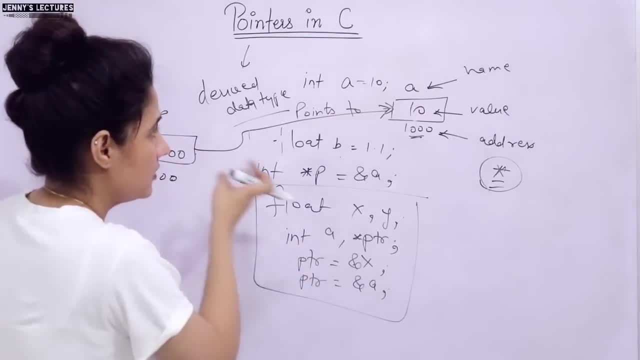 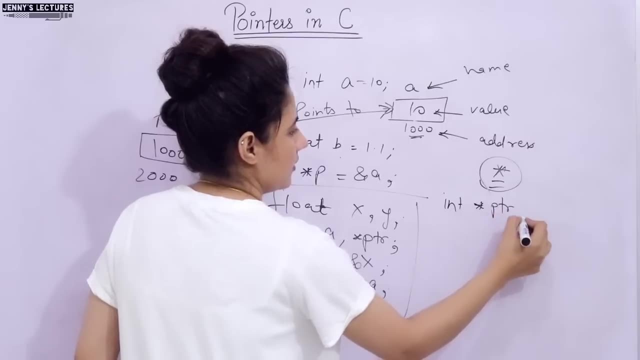 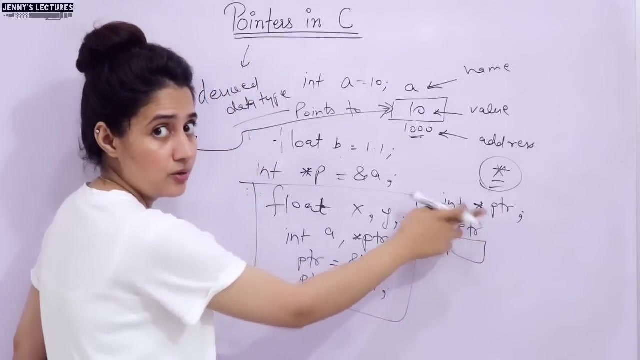 can tell me in comment box: is it correct or not right? so i hope this the basics of pointer you got and see if i write something like this: int asterisk, ptr. so means here we have pointer name. this is a pointer. because of this asterisk we came to know name is ptr, suppose address is three thousand and here 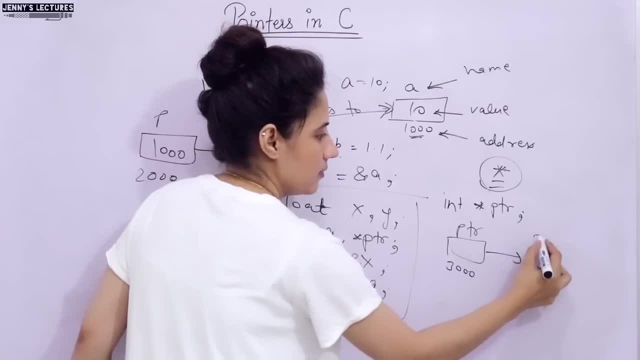 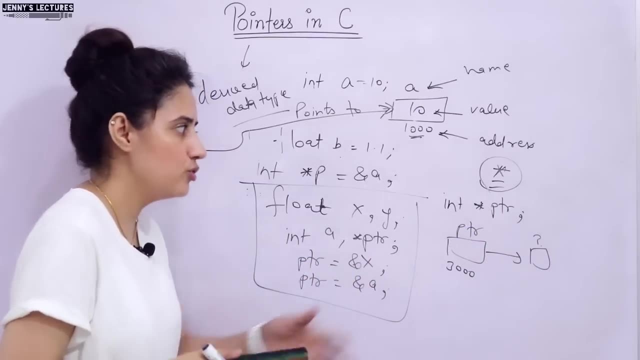 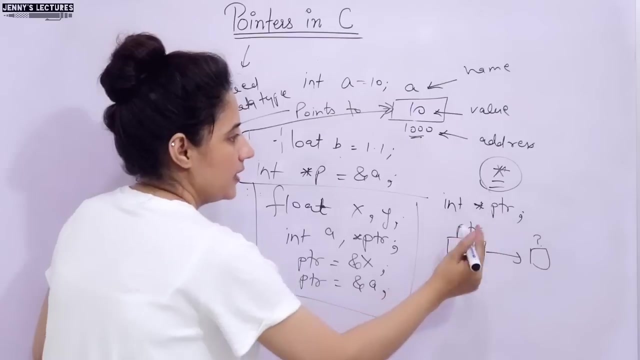 we haven't initialized this pointer so it is going to point some unknown location we don't know. so the these, you know, uninitialized pointers are very risky to use. so before using the pointer we have to initialize these pointers in our program, right? and if you initialize like int, star, ptr, and if you initialize like ptr is equal to address of b. 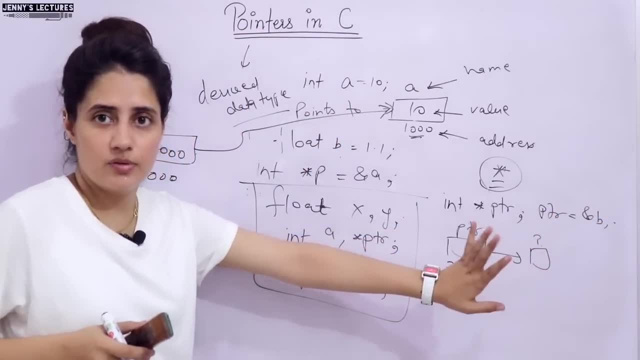 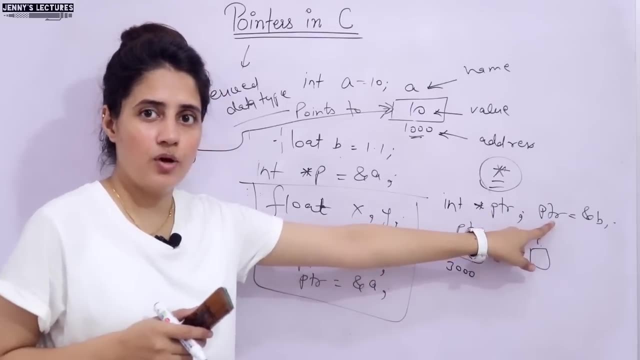 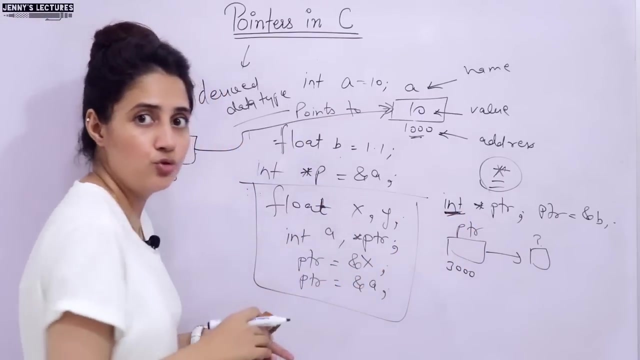 may be, compiler will not detect, will not give any error because of this, but it will give you wrong output. so you have to take care while initializing pointer. you have to take care of the data types, because see b, data type is float right and here it should point to integer data type if you write her. 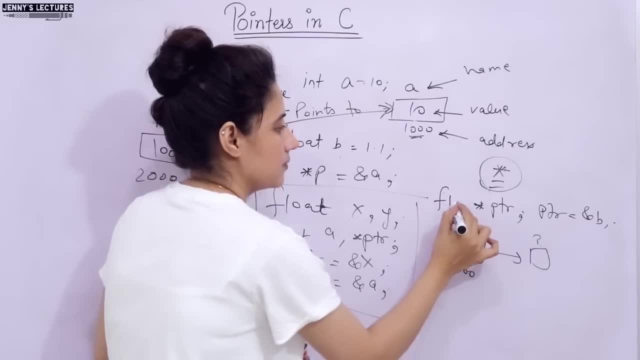 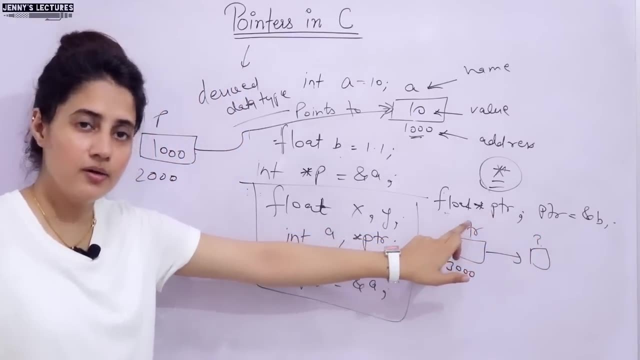 be fine, right? if i write here: float b, sorry, float star ptr, then it is fine. it will point to a variable whose data type is float and b is having flow data type, so it will contain address of b. that is fine, right? so, please, you have to take care about these assignments. you have to take. 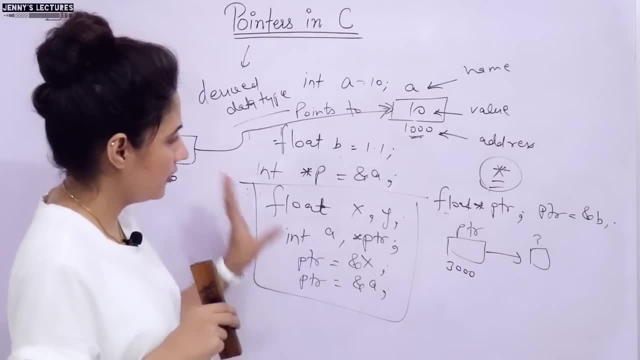 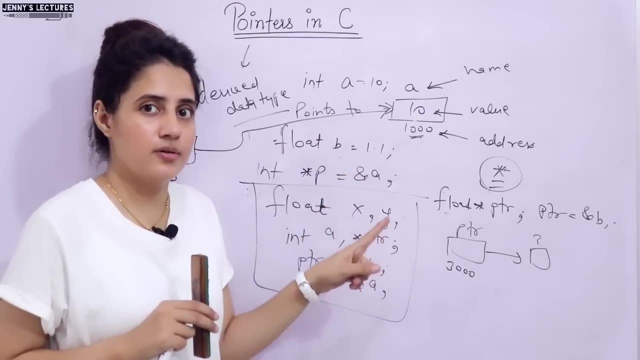 care of the data type also. fine, so now that's it about the introduction of pointer. in the next video you will see some example and some. you know that dereferencing operator and some programs on pointers. so now i'll see you in the next video. till then, bye, bye, take care.